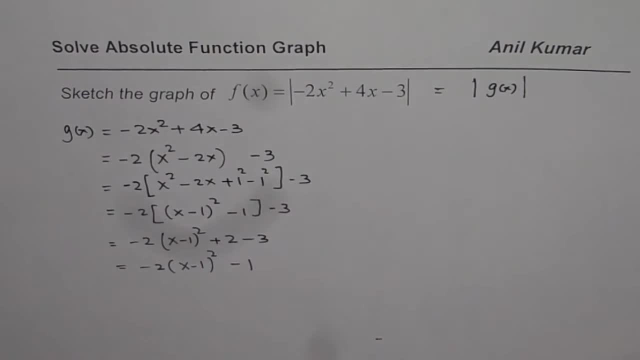 plus 2 minus 3 is minus 1.. So that calculation we get parabola. in terms of vertex. We can roughly sketch the graph here. So what we know here is the vertex in original gehen is: the vertex is at. let's write down: vertex is at 1 minus 1. that is the vertex it opens down right. 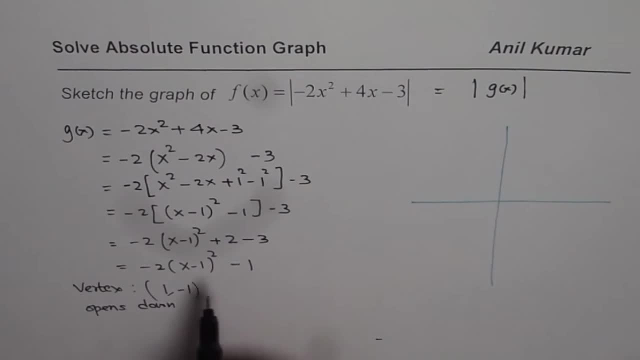 and y intercept, that means g of 0 will be. if I substitute 0 here, I get 1 square minus 2 times 1 is minus 2. minus 2 minus 1 gives me minus 3, right. so that is the value. so taking those values, 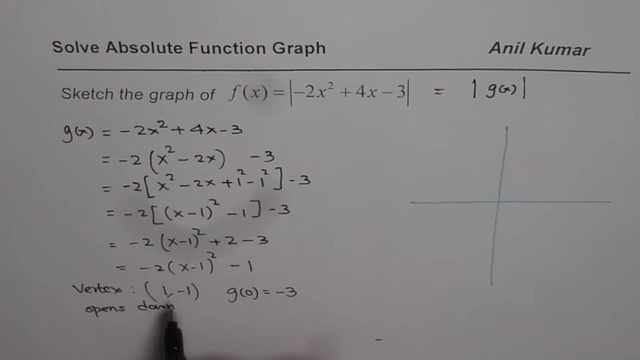 we can sketch the graph, which will be vertex, at 1 minus 1. let us say this is 1, this is minus 1. in that case the graph will be kind of like this: right, so that is the vertex. so that becomes your parabola, which we are saying is the function of the vertex. 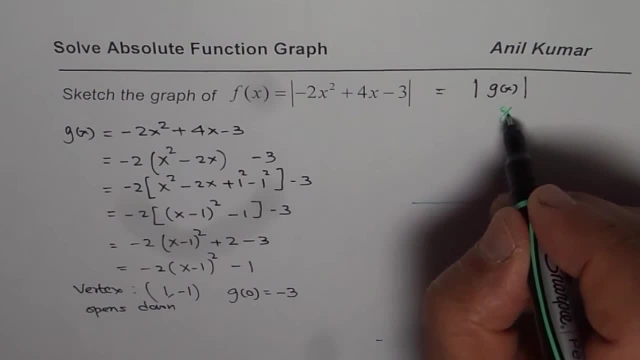 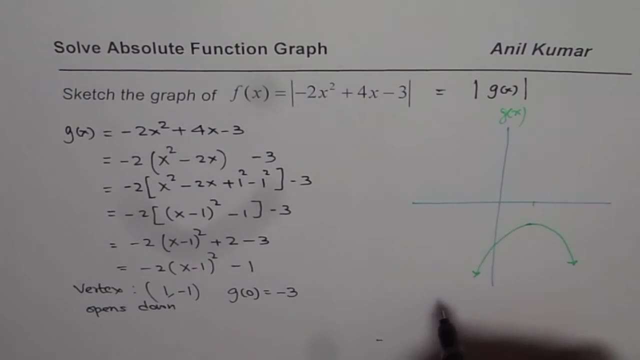 g of x. so this, this is g of x for us. we need to sketch absolute value of g of x. so what we will sketch now is f of x, which is absolute value of g of x. right, that function. so in that case, what happens is we will flip it over. 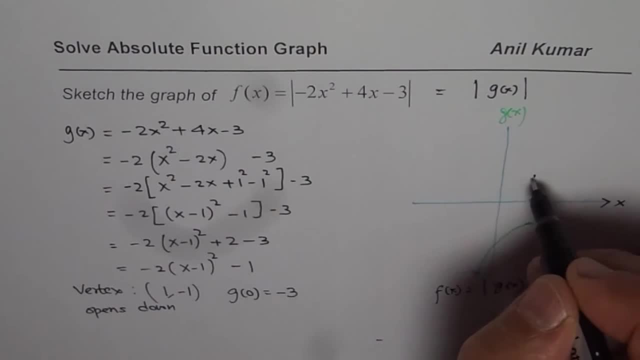 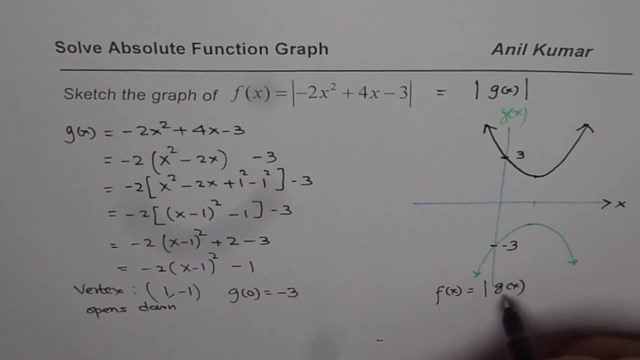 x axis, correct. so this point will appear here. and then this, which is at minus 3, should be at plus 2: three right. so what we get here is kind of a parabola like this, where this point is three right. so mirror image of g of x. mirror being the x-axis gives you the graph of the given function. 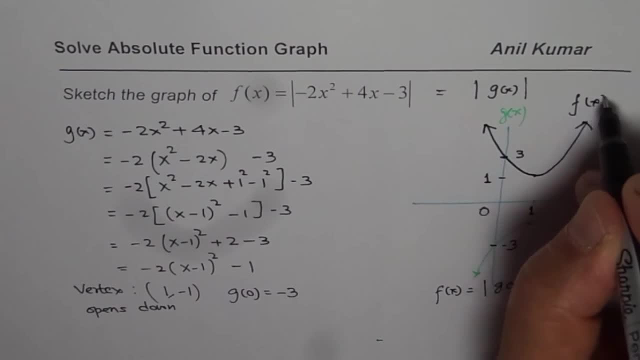 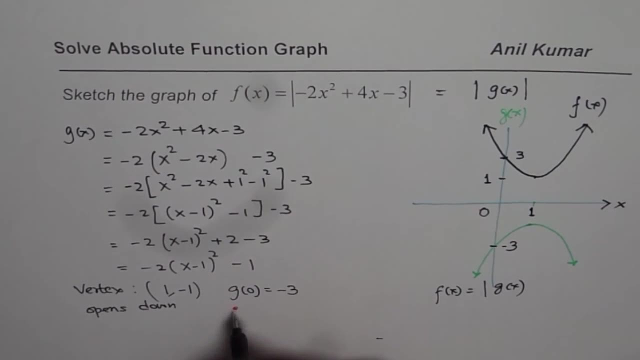 so that is how we will sketch f of x right. so i hope the steps are clear to you. first step: what we did was sketch inside functions. first step is sketch inside function right, which was g of x in our case. and second step was: we need to reflect it.